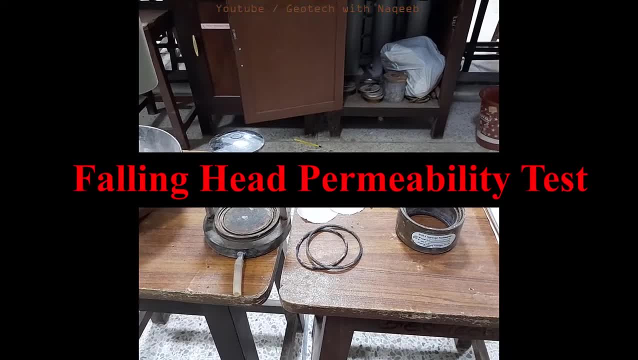 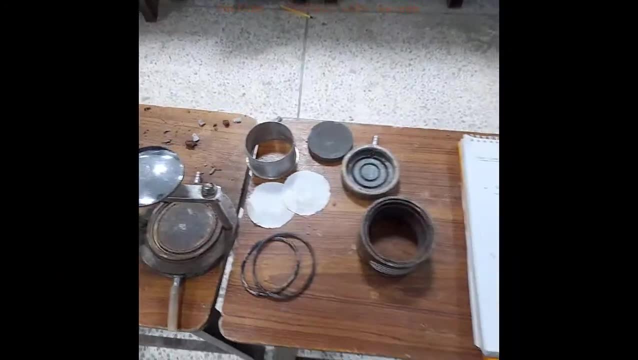 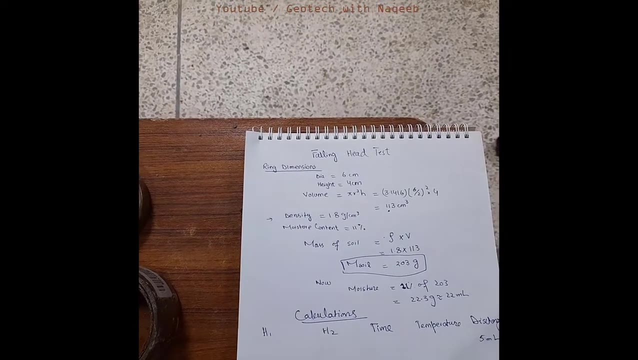 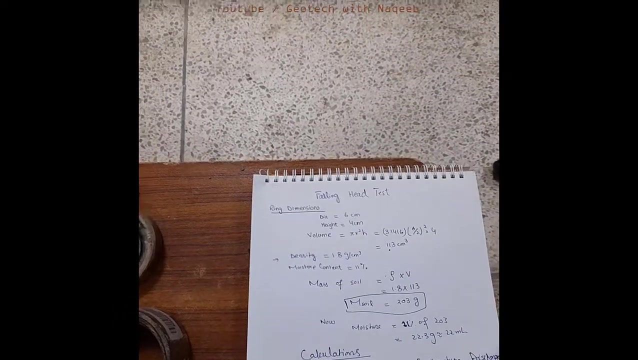 Assalamu alaikum. so now we'll learn how to perform the falling head test, and you can see the apparatus here. Firstly, we need to perform the calculations. We can use the undisturbed sample or we can use the remolded soil sample for this test. So let's say we need to perform the remolded soil sample, the test on the remolded soil sample. So let's have the look at the calculations. 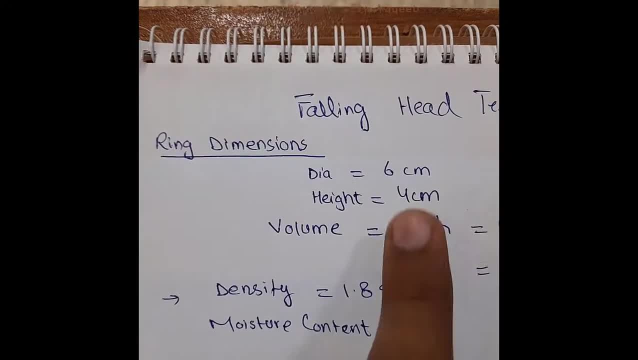 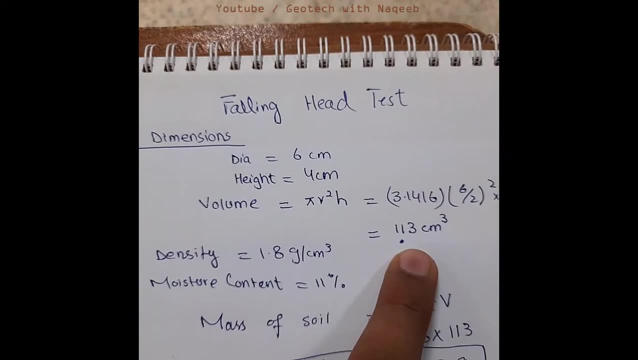 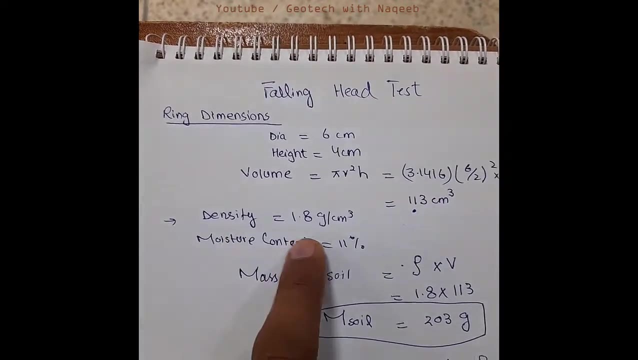 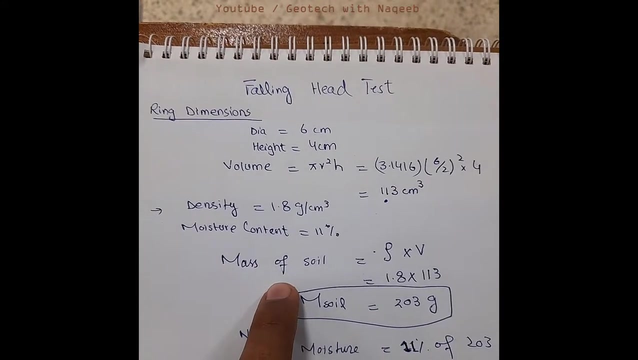 We have the ring dimensions: the dia is 6 cm, the height is 4 cm, and now we'll find out the volume. that comes out to be 113 cubic cm from the formula pi r square h. So now we have the density- 1.8 g per cm3, and we have the moisture content that is 11%. So using these values, we can determine the mass of dry soil required to remold the soil sample, and that comes out to be 113 cubic cm. 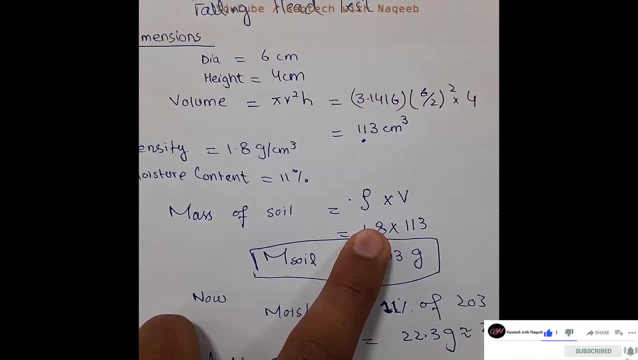 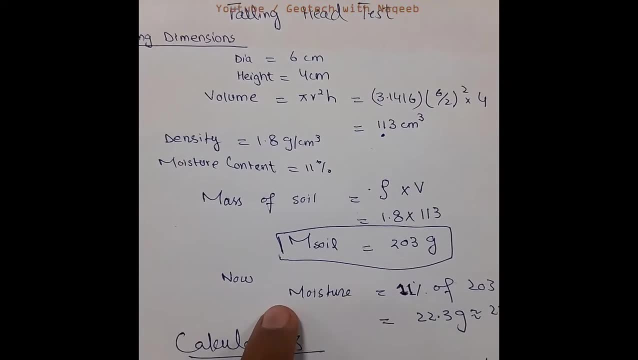 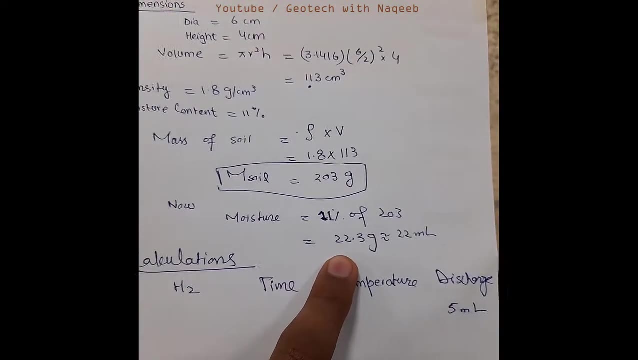 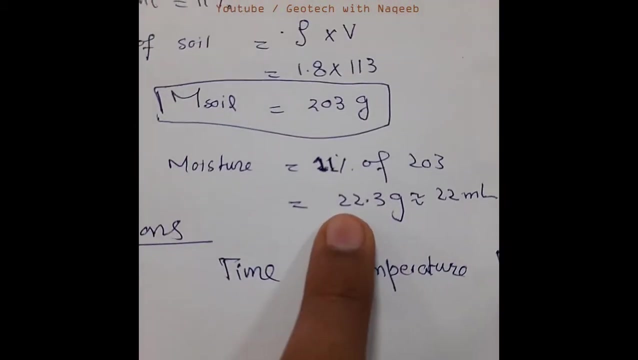 So this much amount of dry soil is required to remold the soil sample for this test. Now we have the 11% moisture content, How much the moisture or water is required to be added in the soil. So this is 11% of this 203 gram soil. So it comes out to be 22.3 gram, or it is equivalent to 22 ml. 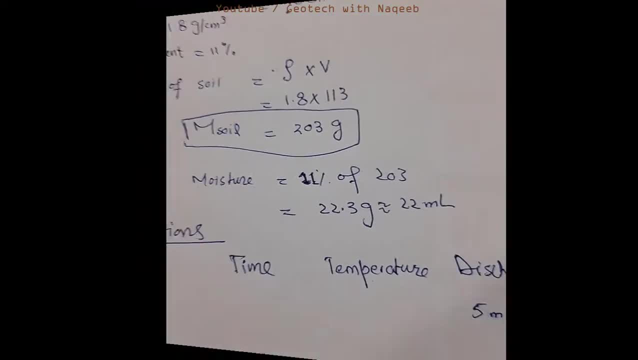 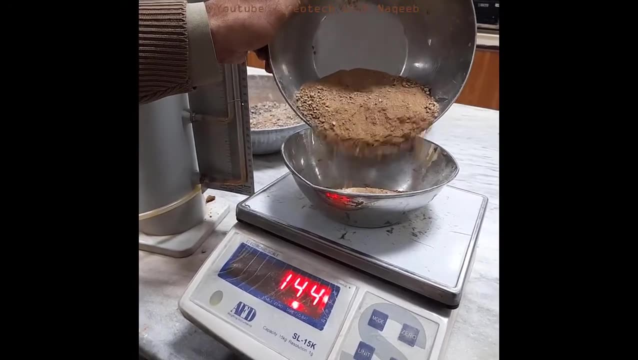 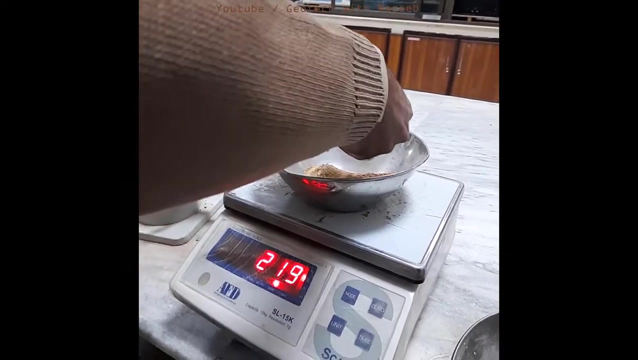 this much amount of water to prepare the soil sample. so have a look at the soil amount. we have to take 203 gram of soil. this test is basically used to find out the hydraulic conductivity of fine type of soil. so we'll take fine type of soil here. 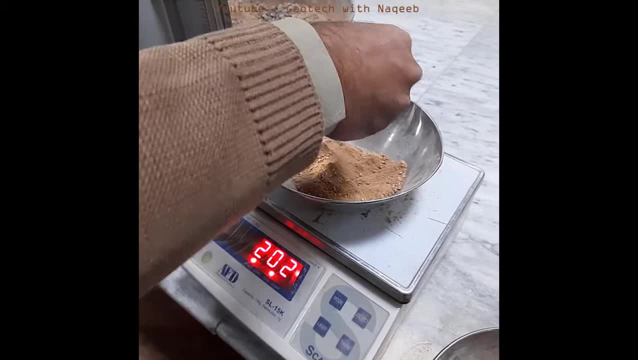 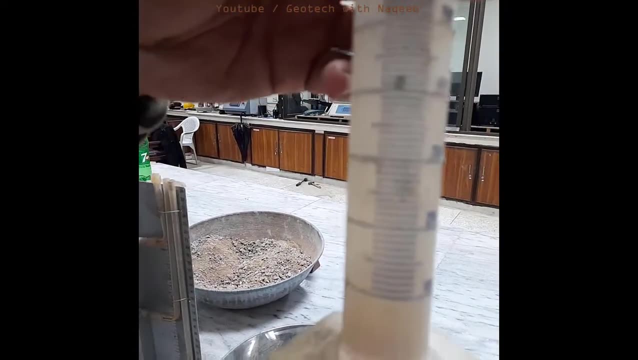 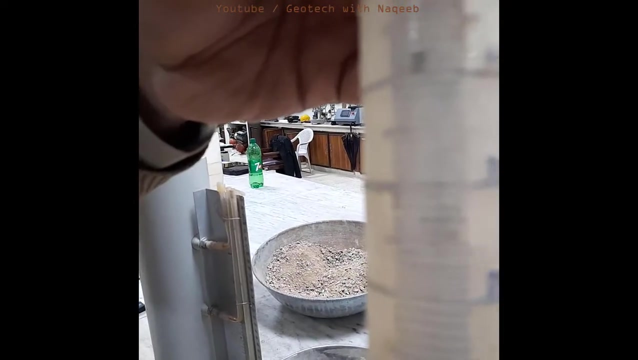 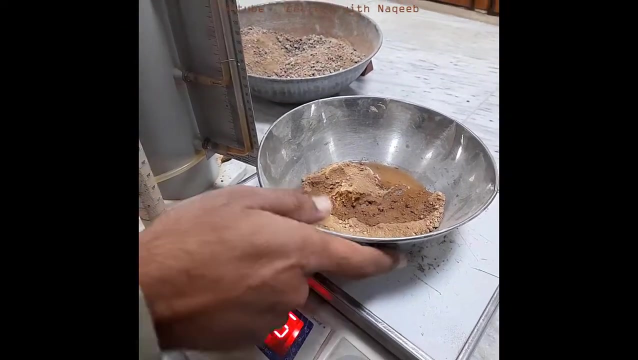 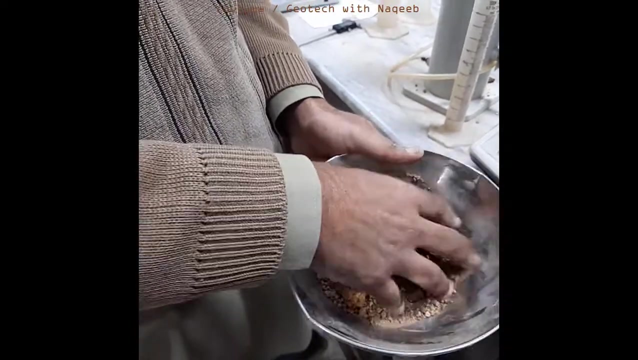 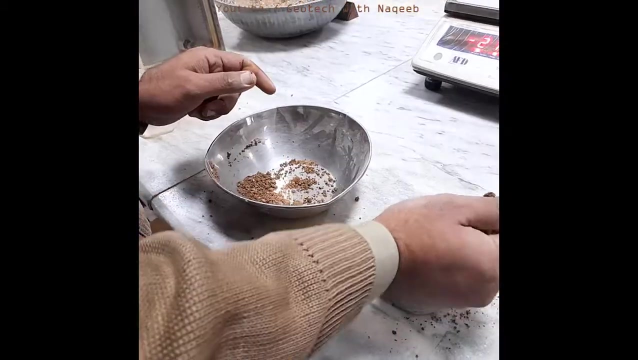 203 gram. now we have the water. the equivalent amount is 22 ml. you can see here the graduation is 22 ml. yes, now we'll add this water in the soil to remove the soil sample. basically, we'll mix it thoroughly. so now we will place this prepared soil sample in the mold. 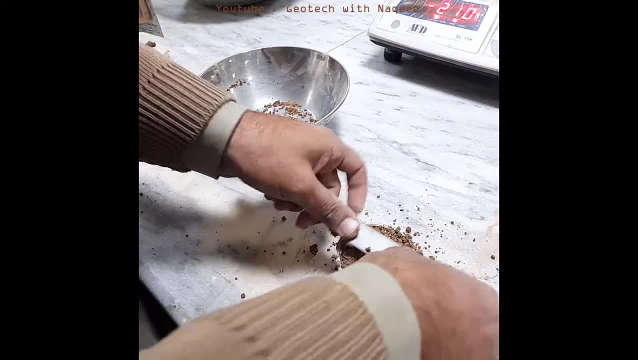 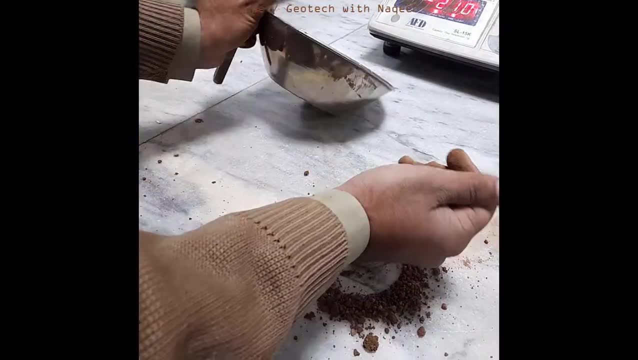 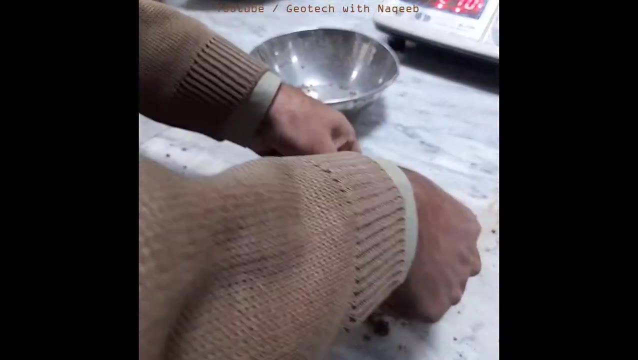 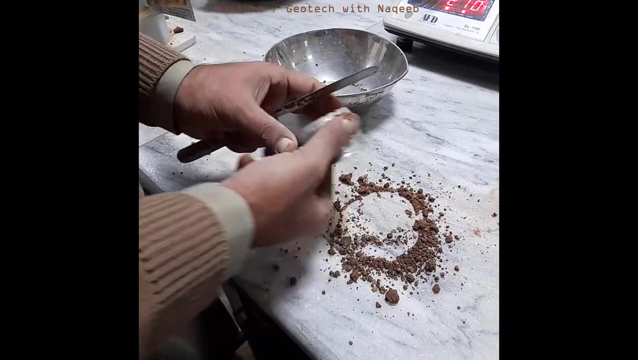 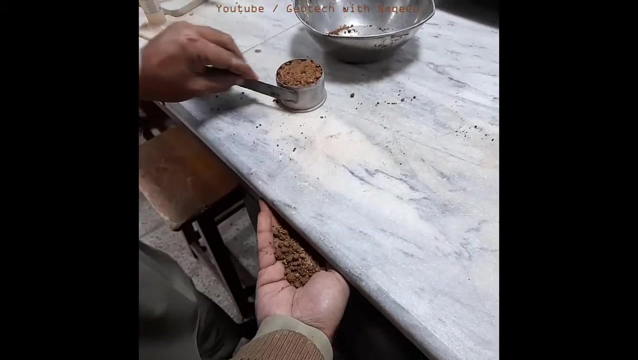 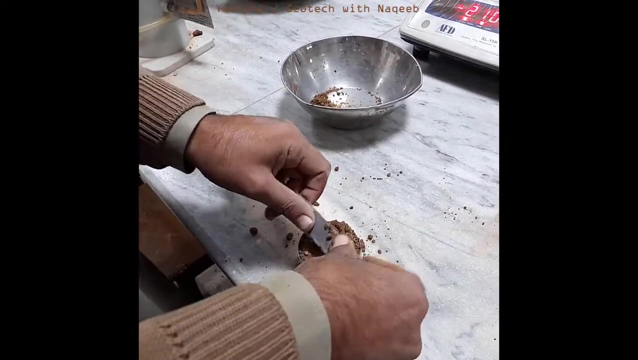 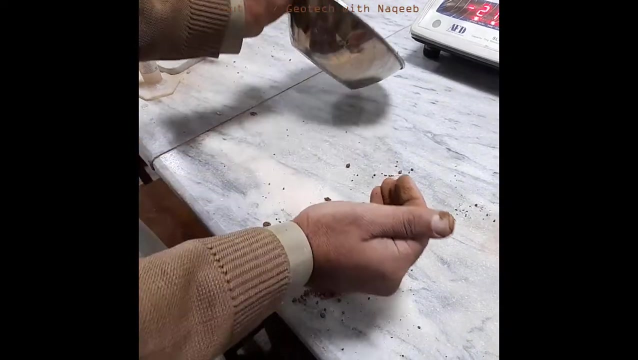 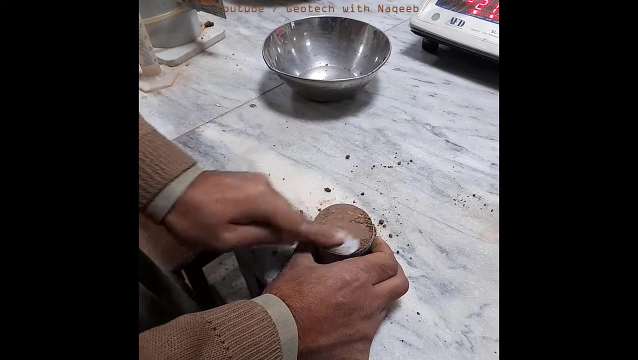 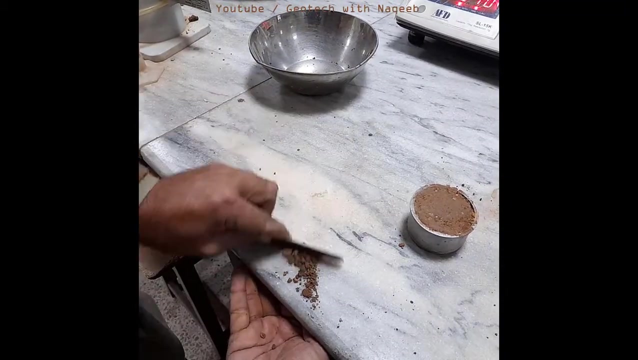 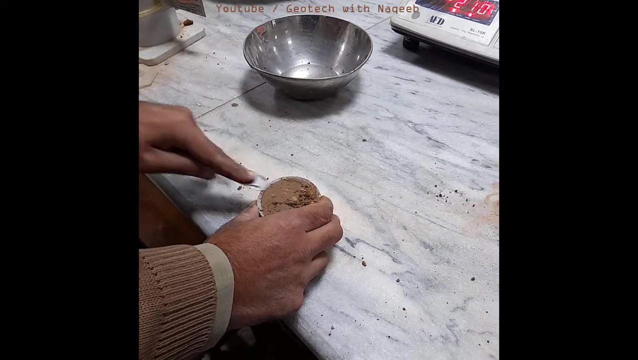 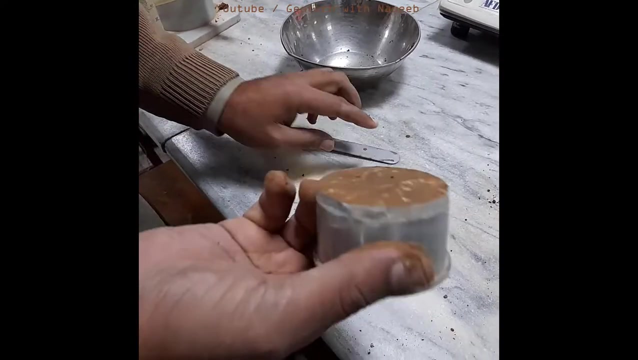 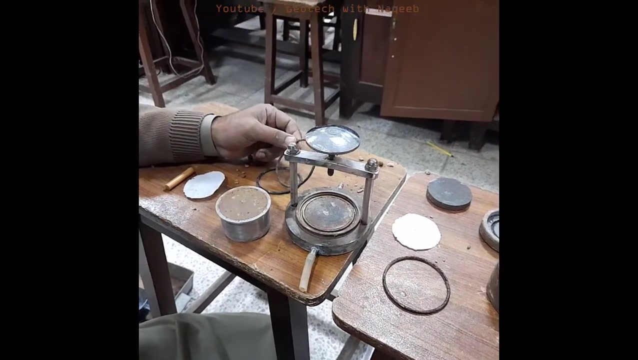 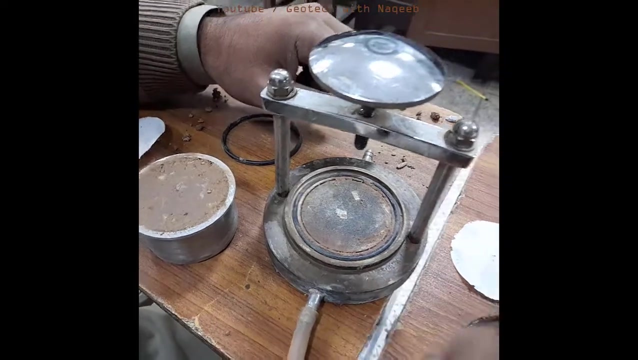 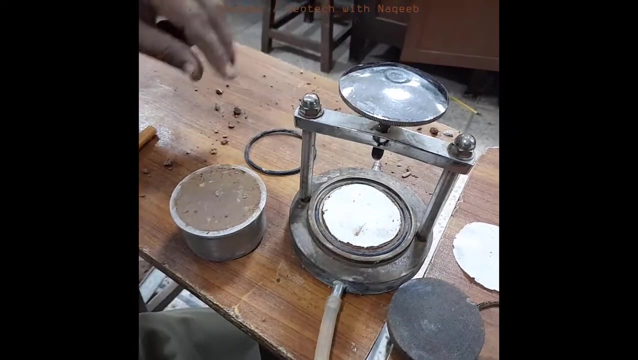 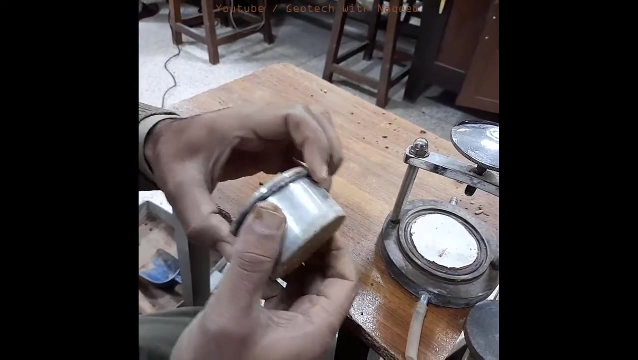 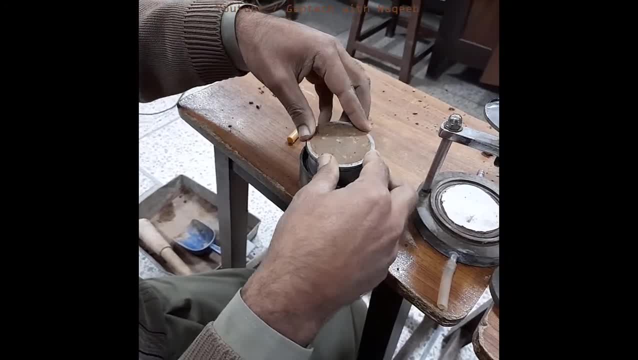 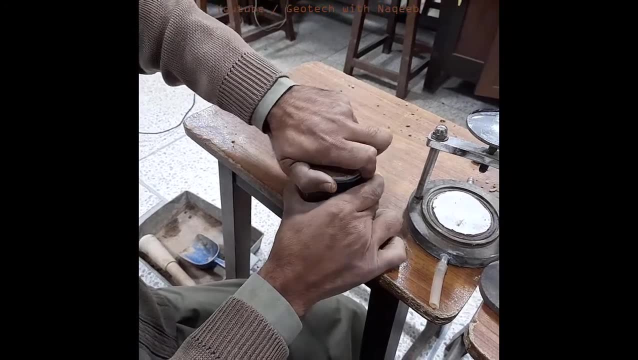 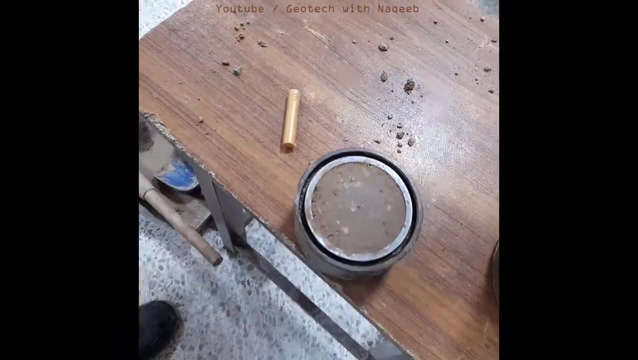 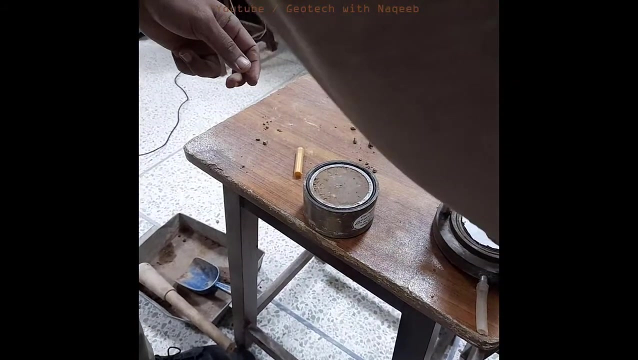 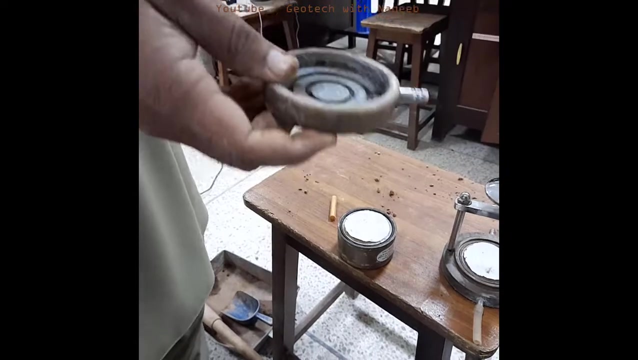 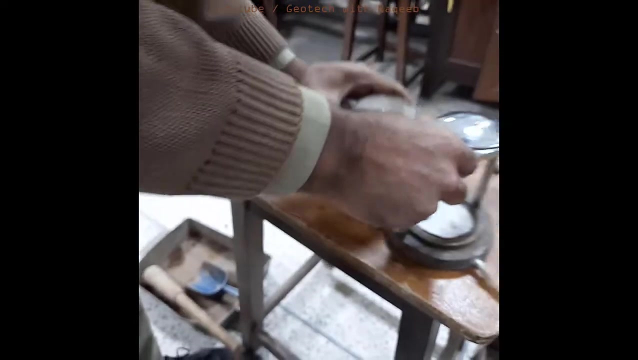 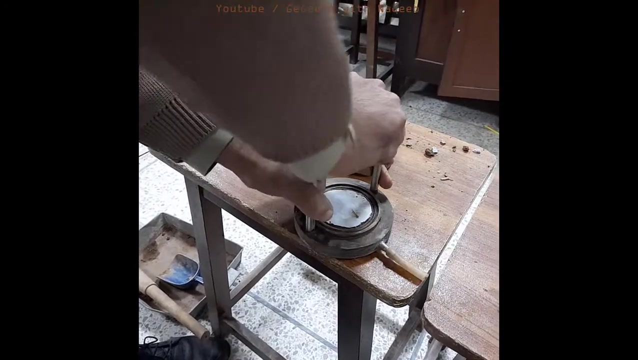 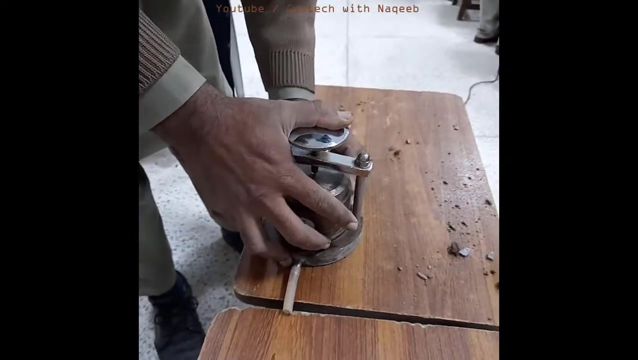 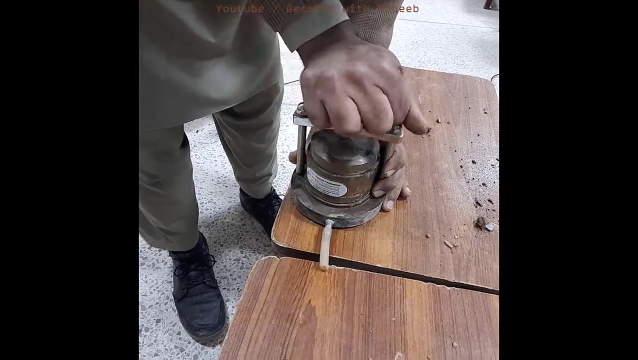 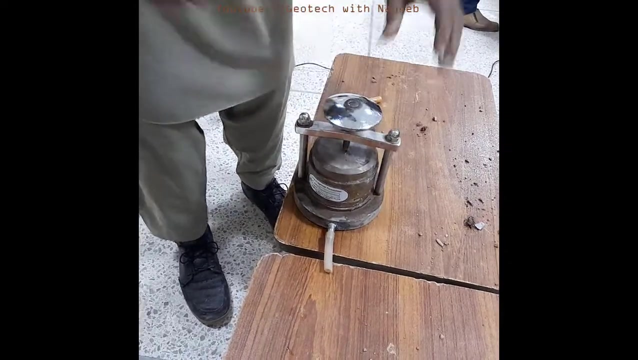 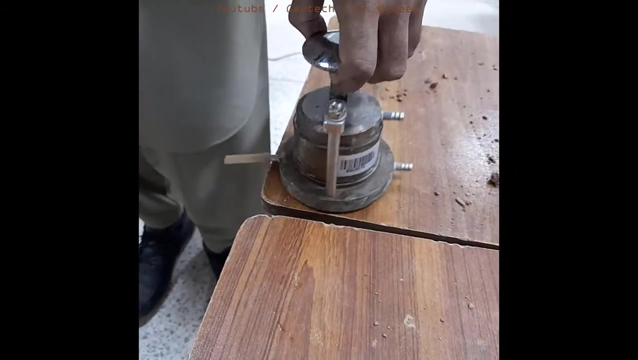 so, so, so, so, so, so. so how will place the sandstone and will close this assembly? we place- it was the base plate- just to fix it. okay, now the assembly is ready. so this is how we basically assemble the apparatus. now we'll have to perform the test to determine the hydraulic conductivity of point up of side. 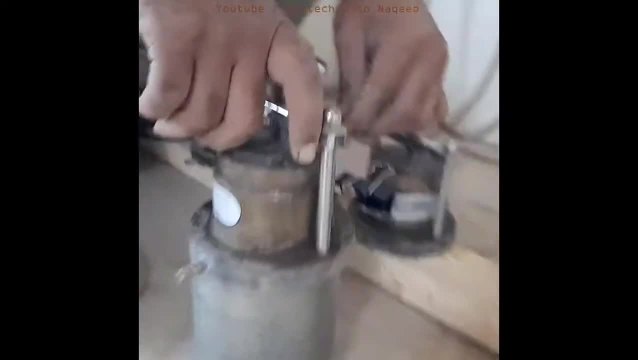 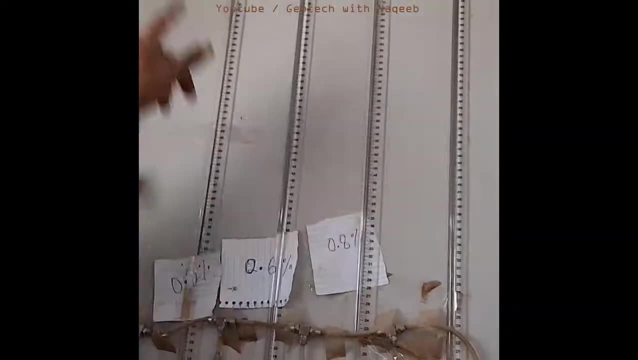 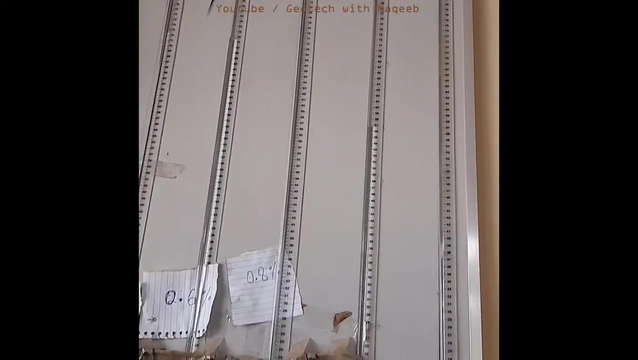 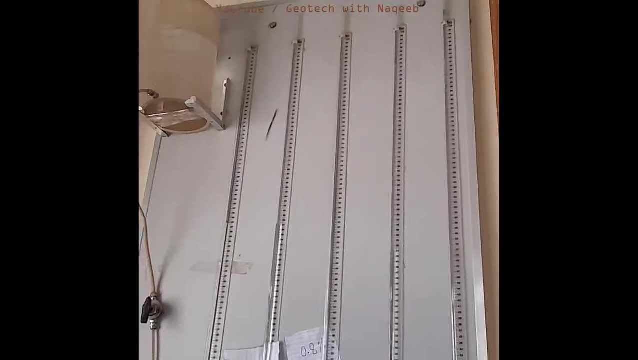 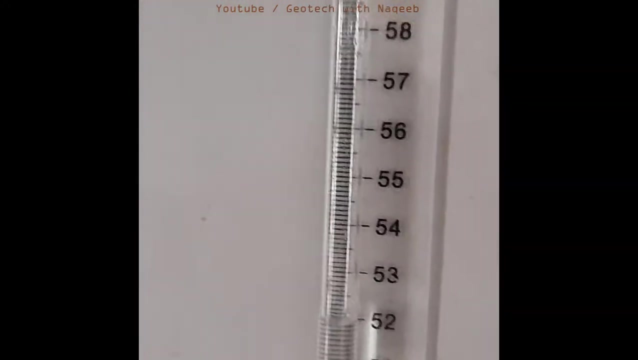 no, firstly, will saturate the soil sample you can see, will attach it with the razor wire. and here you can see the periods: five burettes and the tank, the story tank of water and five burettes. it means we can conduct five tests at the moment and this is the pretest you can see now. so we 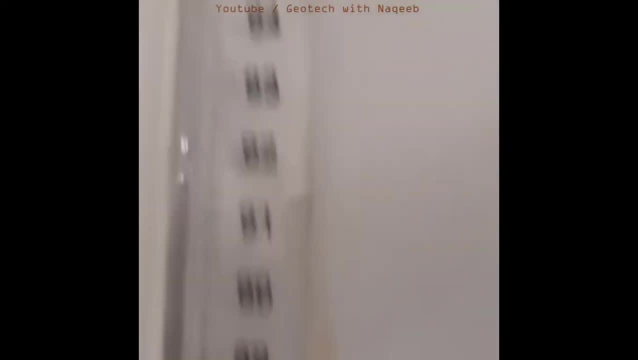 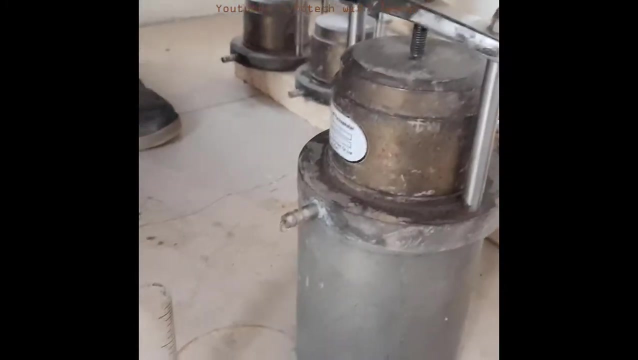 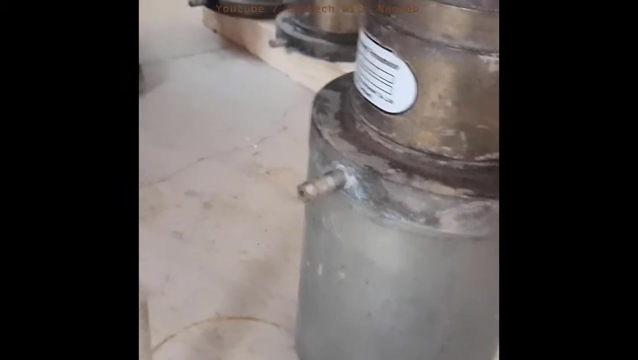 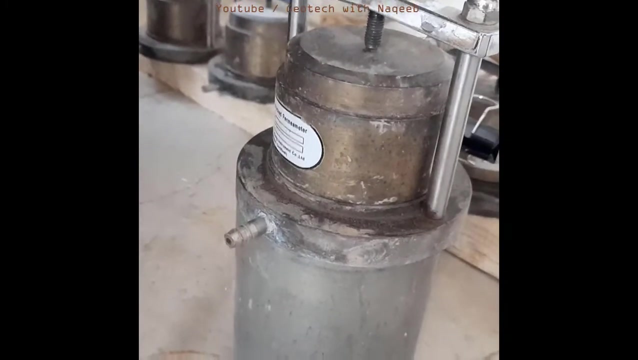 have the 40 centimeter head that will be added in the calculation in h1 and h2. now we'll saturate the soil sample. now we need to check how we will check the saturation stage is completed. when the water starts flowing continuously from this from here, it means the soil sample is fully saturated. so now we need to take the values. 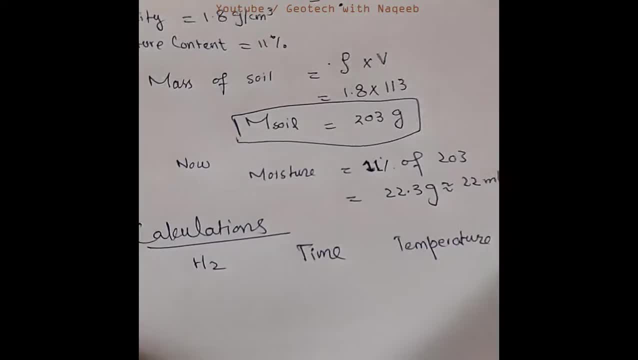 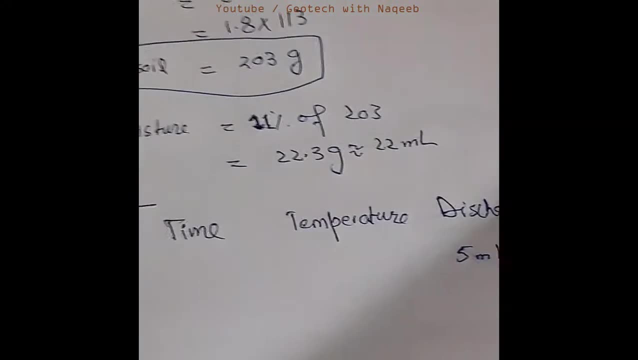 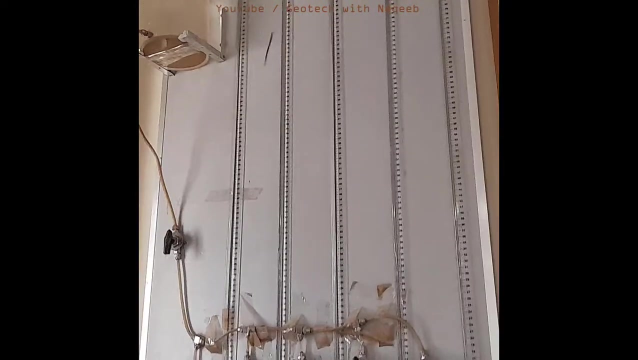 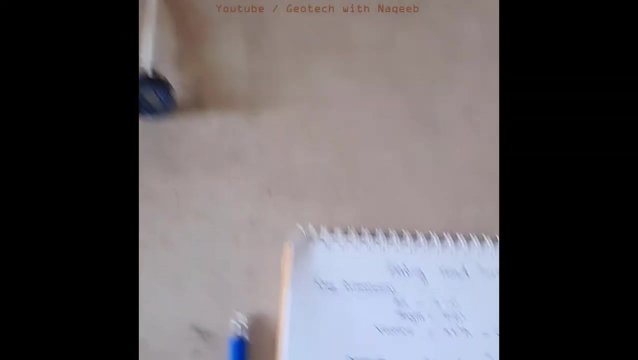 of the observation will firstly determine h1, h2 value, then time, temperature, and we have the fixed discharge value, that is 5 mm. we have to collect 5 ml of water and we have to note it down, the time and the difference. so let's see now. firstly we'll note down the h1 value and then we'll 4.5 for 94. okay, so, 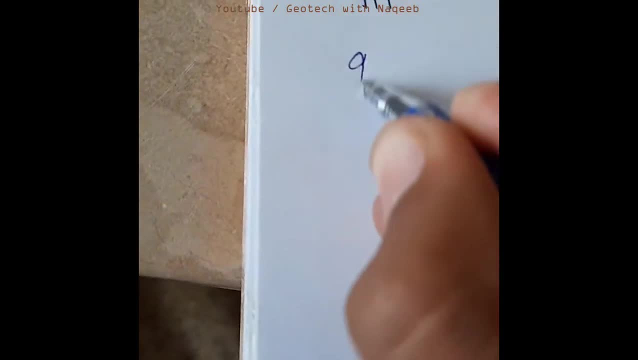 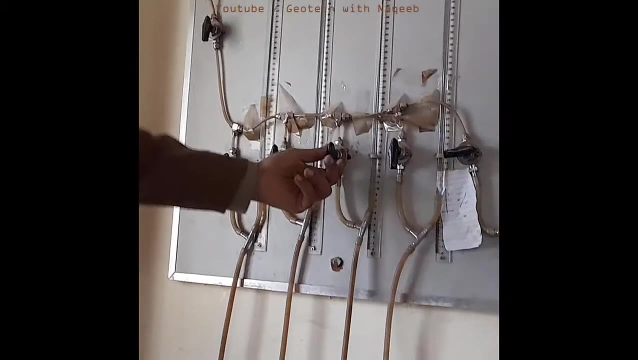 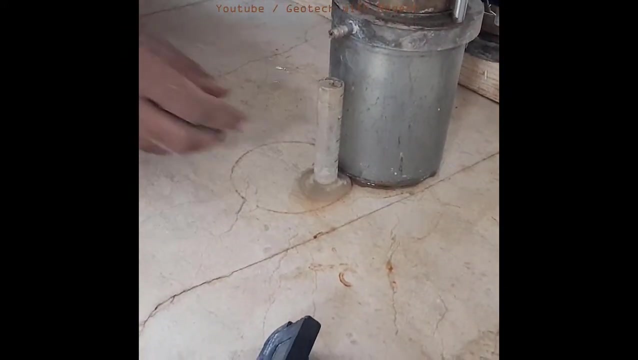 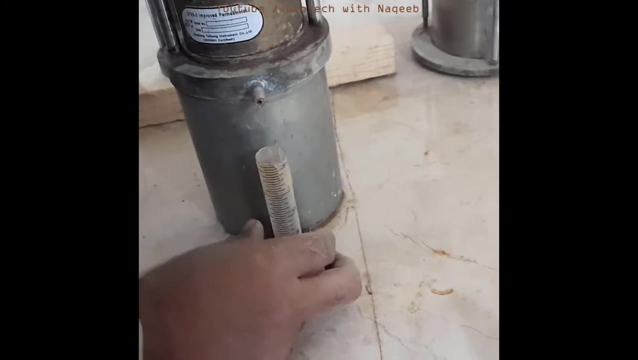 ninety four point five is the h1 value. ninety four point five centimeter is the h1 value. now we'll close the razor wire and we'll start the test. and now we'll start collecting the discharge and we'll note down the time. now we have the fixed discharge value, that is five ml. 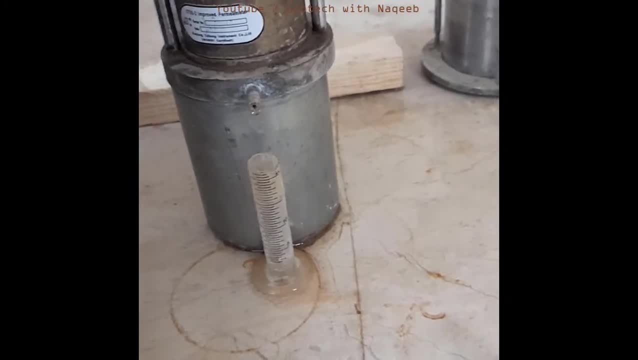 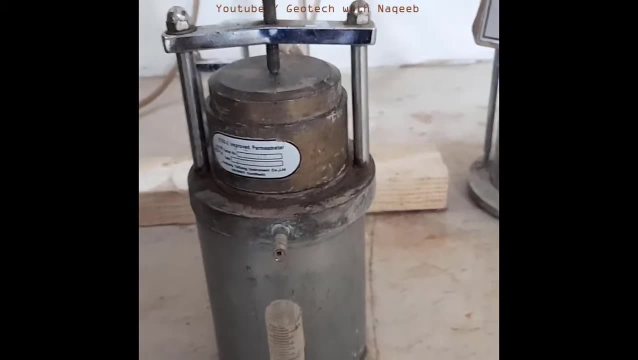 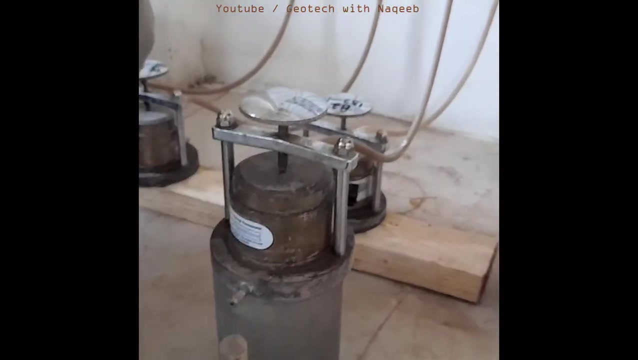 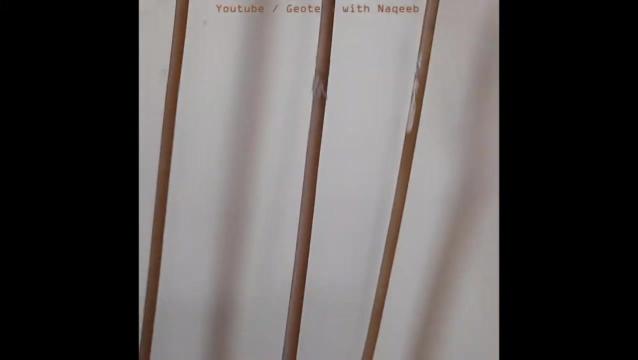 and we have to note down the time that- how much time it will take to fill or to collect the five ml water from the soil sample. that is the representation of the hydraulic conductivity of this soil. now the important point is the ��기는 ability of the moisture in this columbine about, and you have to consider all the sample size. 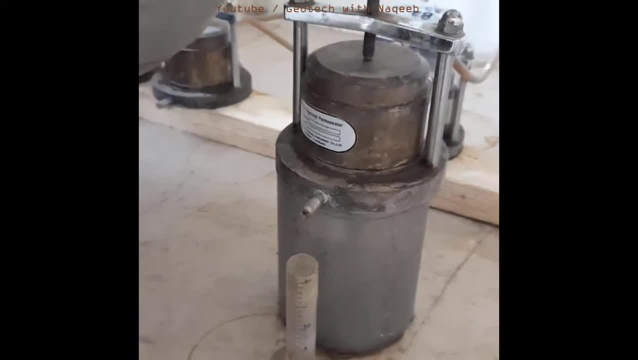 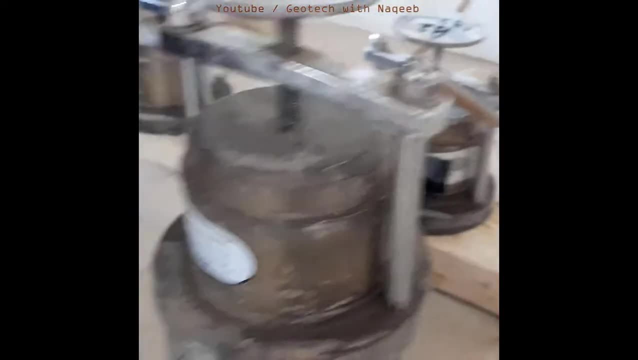 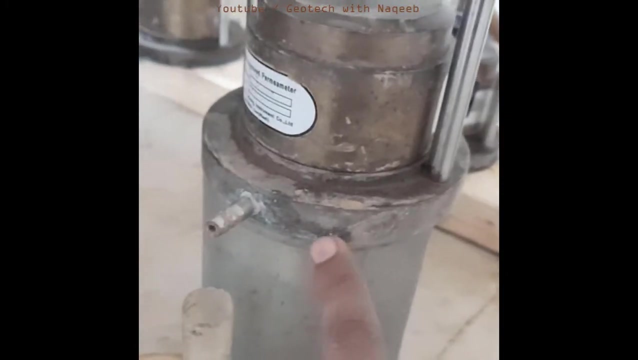 all samples are commensal, so all one sample need to have about 10 bit more Than before. if the say so, are these things starting from 0? but oil soil samANTHA is 40 centimeter down from the burette so will have to add this two centimeter value in the calculation phase. so most 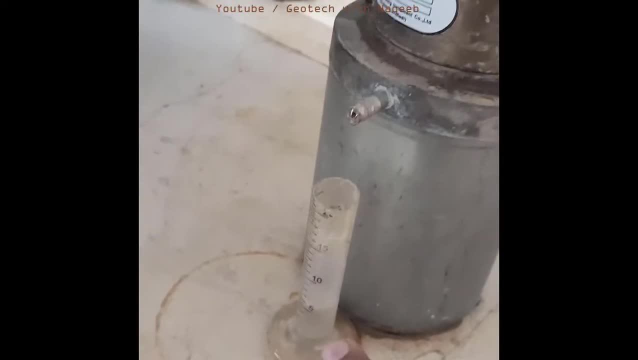 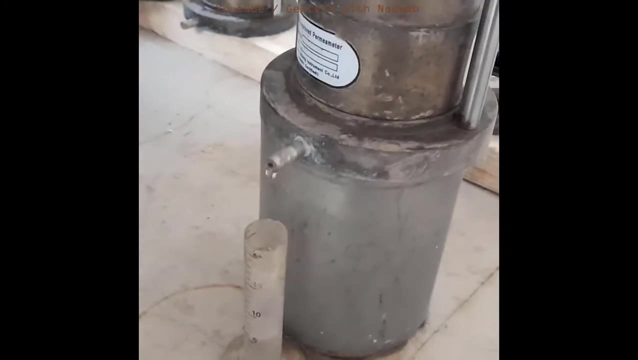 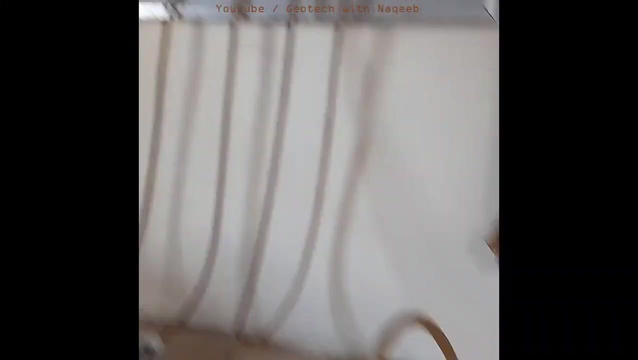 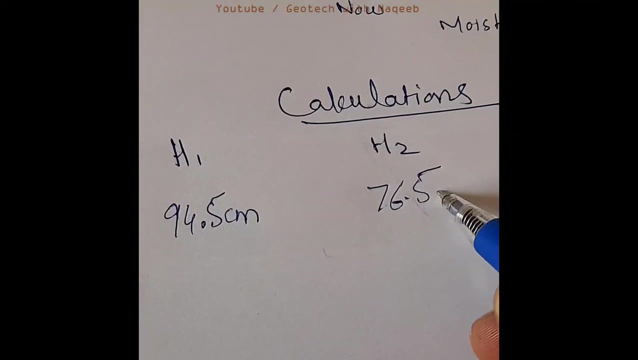 importantly, you can see, there is not any kind of leakage from the, just a slender, nothing else. it's just. we have provided a base. so now the 5 ml discharge is complete, you can see, and the h2 value is 76 point 5 time is 2.